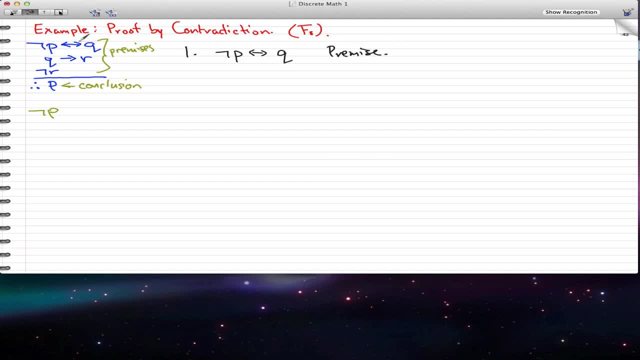 And that is our premise, And we have used our first premise. So our second step is we're going to try to break that first premise down, And it's going to be broken down like so: Negated P implies Q And Q implies negated P. 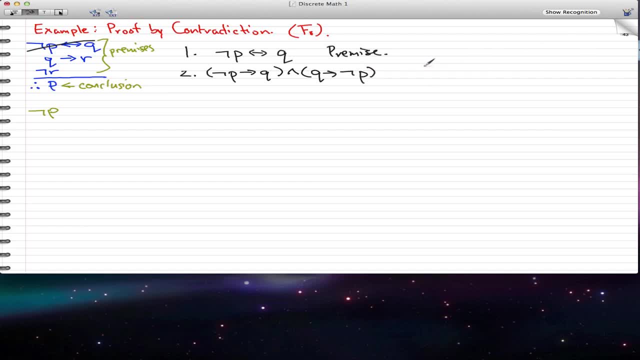 So this is from step one And this is from the rule that when we have a biconditional, we break it down. It's pretty much logically equivalent to- and I'm going to write that down here because I don't think I have enough space- It's going to be logically equivalent. 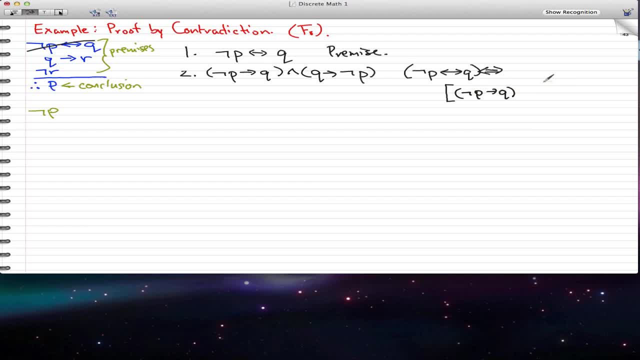 to: negated P implies Q And Q implies negated P, So we broke it down to this form from that rule. So then we have our third step, And our third step is: Negated P implies Q, And this is taking step two and applying the rule of conjunctive simplification. 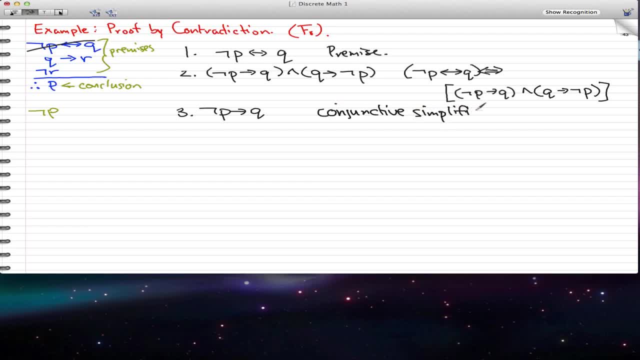 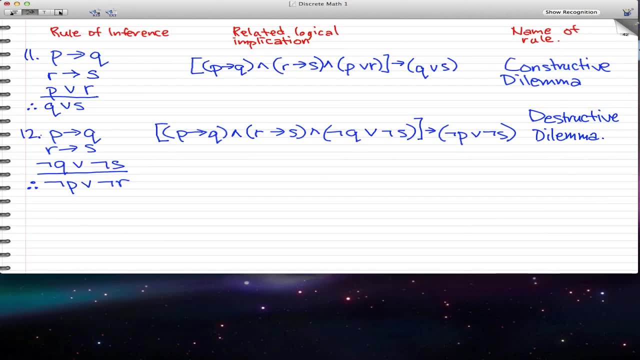 And this is one of those rules that I have not went through with you guys, And if we just take a look back to find it, it's this rule here, number seven. So, going back to where we were, we just apply conjunctive simplification to step two. On. 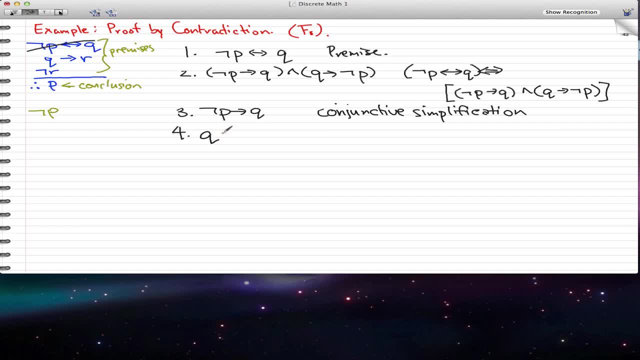 to step four. Now, step four: we're going to take care and use another one of our premises, which is Q implies R, And this would just be a premise. And our fifth step is: while we have a negated P implies Q, Q implies R. Well, that is pretty. 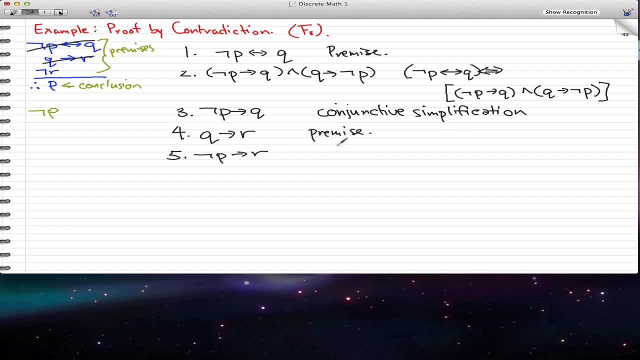 much. just negated P implies R, And that is from the law of syllogism And we know, or we are very familiar with that. I know that we are. And next we have negated P, And this one is the premise that we assumed, The premise that we assumed So far, so good. So this is 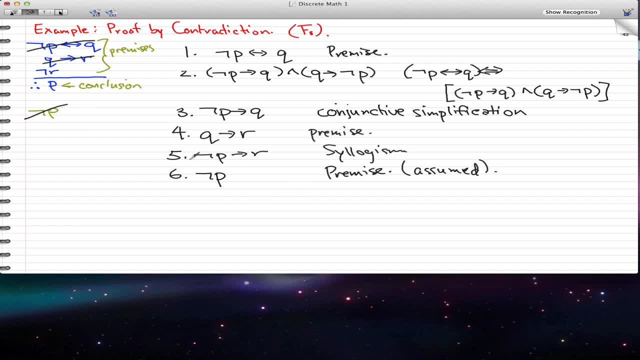 the premise that we assumed And we have, negated P implies R and negated P. From that we can use the rule of detachment or modus ponens to get R. So modus ponens, The eighth step is we're just going to apply our last premise: negated R. This is our premise. And nine: 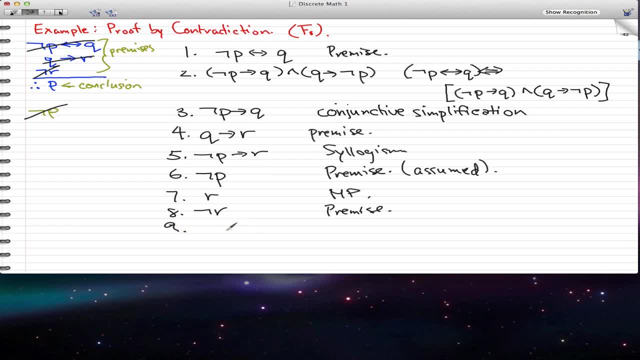 we have For nine. we have R and negated R And we know that this is pretty much equivalent, or logically equivalent, to false. So that is one of our inverse laws from the laws of logic. So that's how we got our FO. So what we set out to do is we set out to use these four. 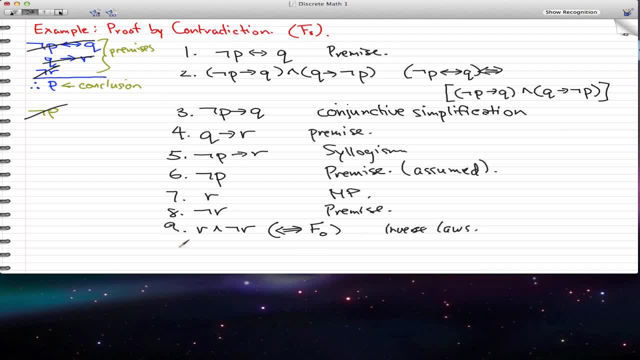 premises to derive a contradiction FO. And we did derive a contradiction FO. So ten, this implies P, And this is by using a negated P number six and nine to get P, And that is by the proof of contradiction. 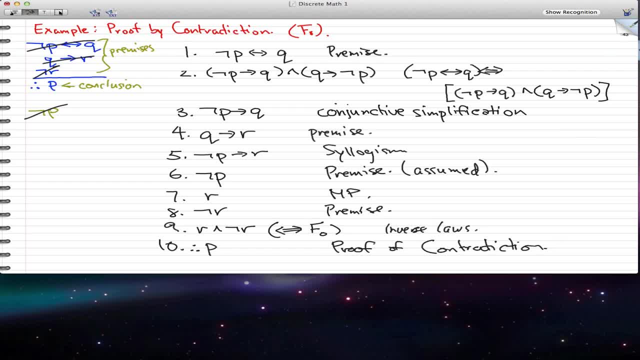 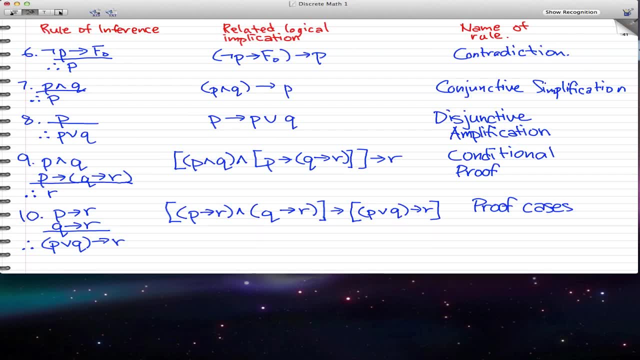 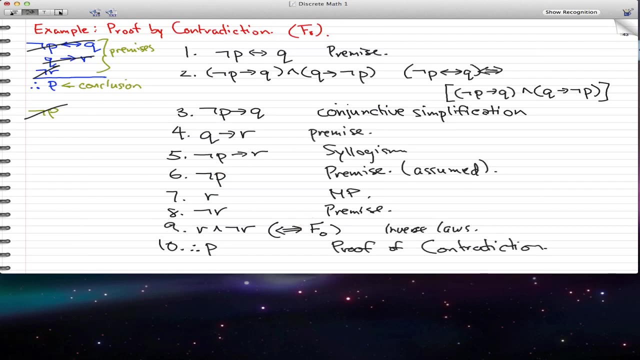 Proof of contradiction, And again, that is from one of our laws here: Negated P implies Negated P implies F-O implies P. That is contradiction, because we have our negated P and we have our F-O. So what I want to do now is I want to explain what happened. 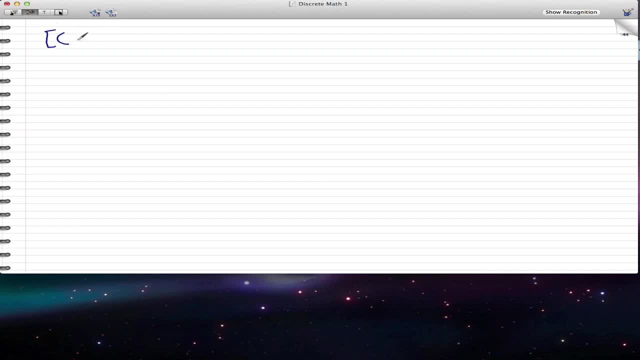 So this is what we found in the end. We have our three premises in the beginning, which is like: so? So that's our first premise, This is the second premise that I'm writing out right now, And negated R is our third premise. 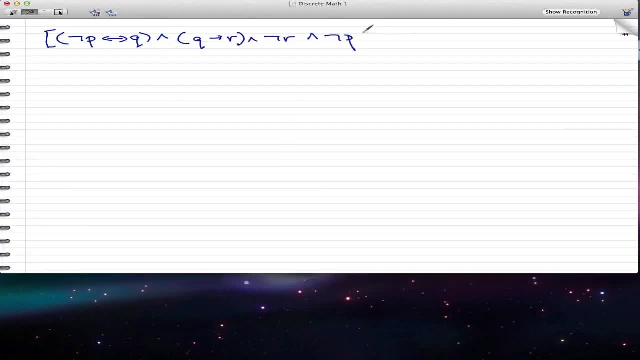 And we have our assumed premise, which is negated P, And what we found is that all this implied false. Now, because our first three premises are given premises, they will have the truth value of true or 1.. Now for this whole statement to be false.